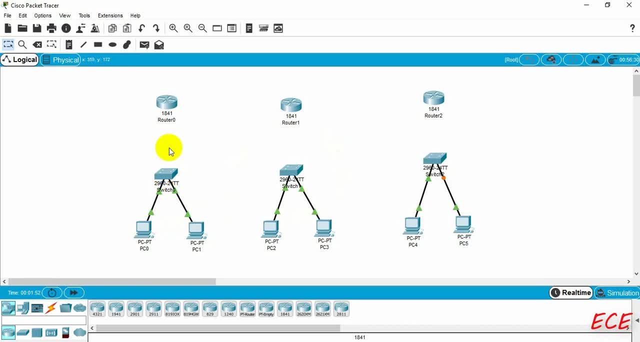 you. here also, we are using copper straight-through wear and we will connect routers if fast return at 0. here you need to remember it because you will need to configure the router with the IP address that will be same as the end devices IP address, that we will create a network that have same IP address, same 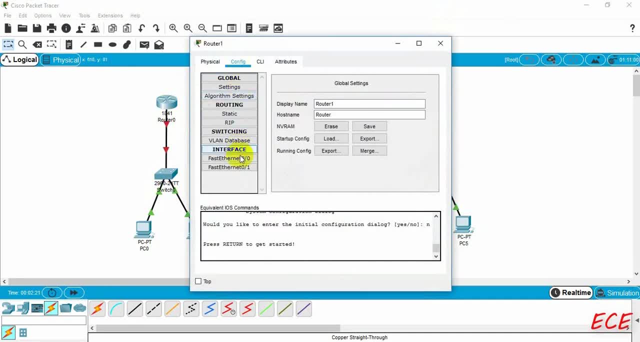 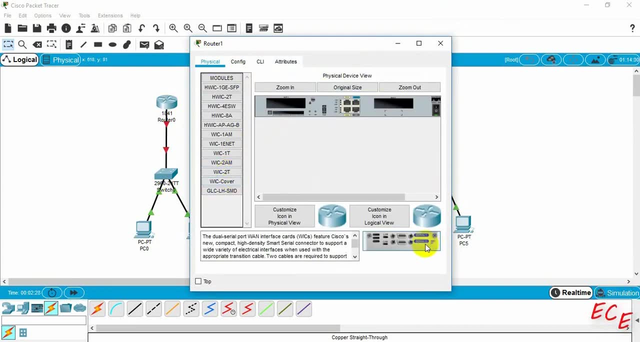 net ID. Now we need to. you can go to configuration and see that there are only two port. we need more than two port to connect three router. So for that we need to go to physical and then WYC2T and turn off the switch and take. 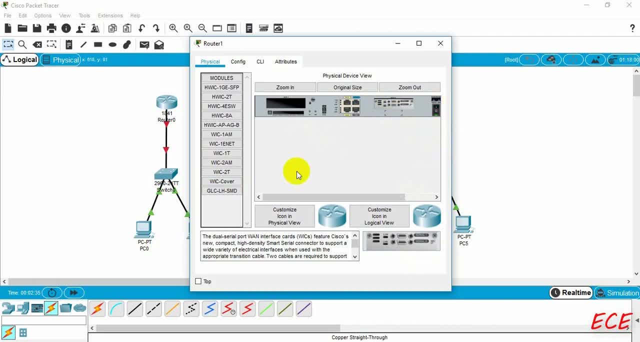 this inside this box and then turn on the switch again. You can see that device is booting. so let's just do this for the other network And after that WYC2T again turn off the switch, take it inside the box and turn that switch. 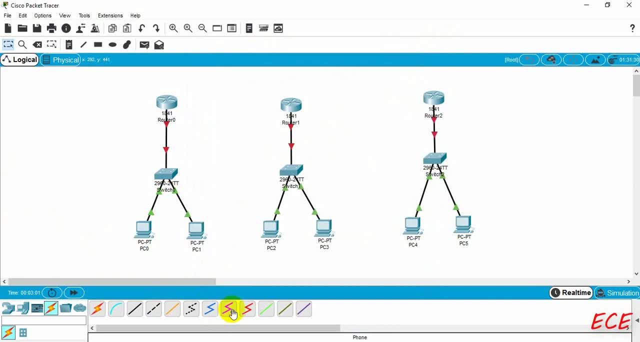 on Now everything is ok. so we need to connect them, as this is our serial port, so we need to connect with serial wire. So here, serial port 0 to serial port 0, we are connecting with serial DTE line. Here, serial port 01 to this router, serial port 0. 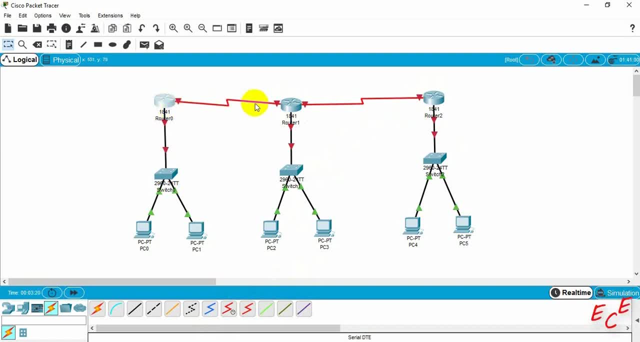 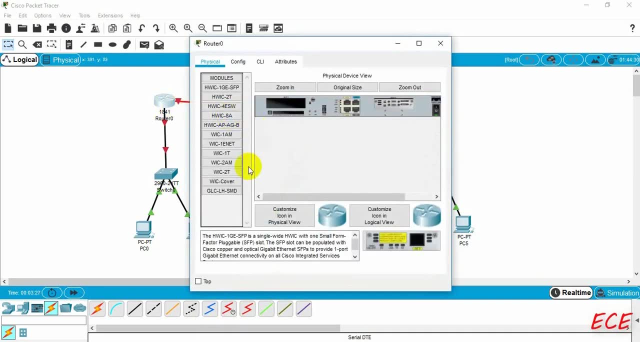 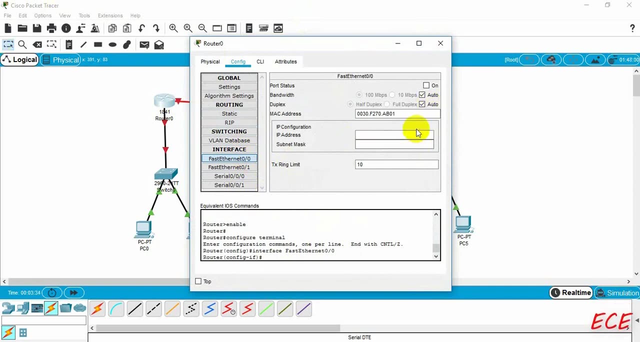 Ok, And now we just need to rearrange them a bit and then configure them. For configure them, we need to give them IP address. for that, go to configuration, and here we need to give the IP address. That is why I was saying that you need to remember them where you are connecting the. 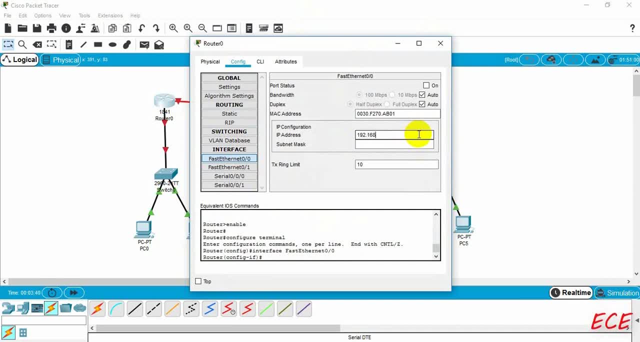 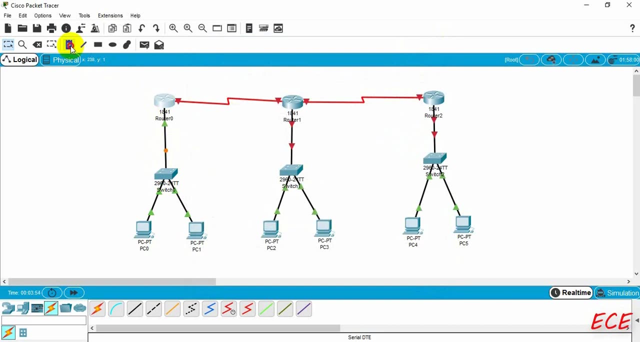 routers which port to which side? Here we will give this IP address: 192.168.1.1.. Here our. I am using a class C IP address Here, as you can see, And then turn on this router. You can see the green signal. so this line is on. 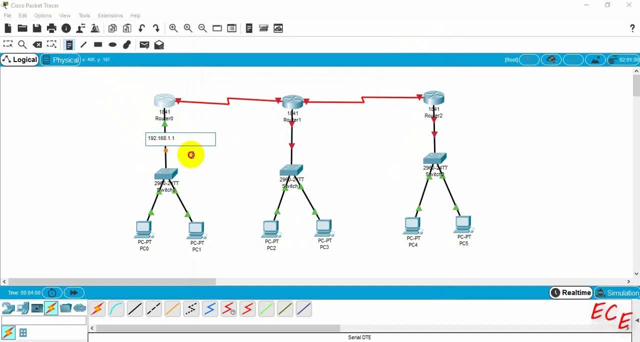 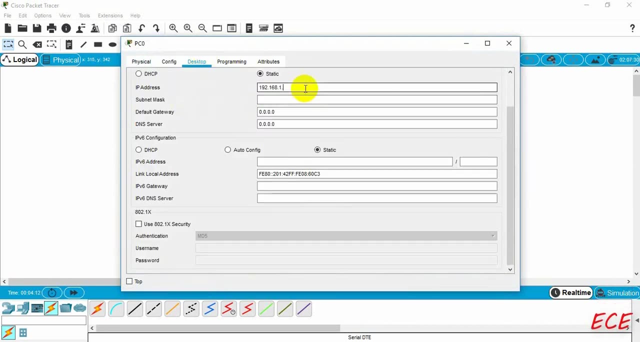 Let's take a note so that we don't forget this IP address. And now we need to have the same IP, same net ID in this whole network. So we need to have the same net ID and the host ID will be different. So we can add from 0 to 255 devices. 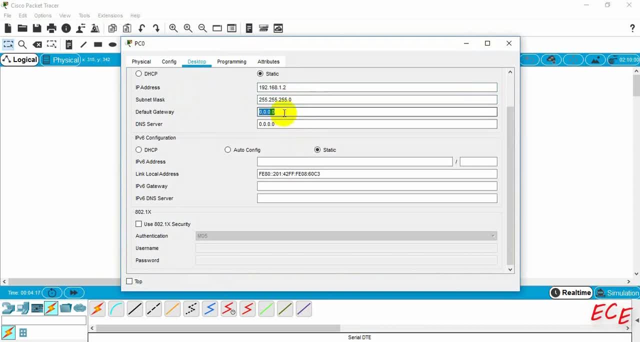 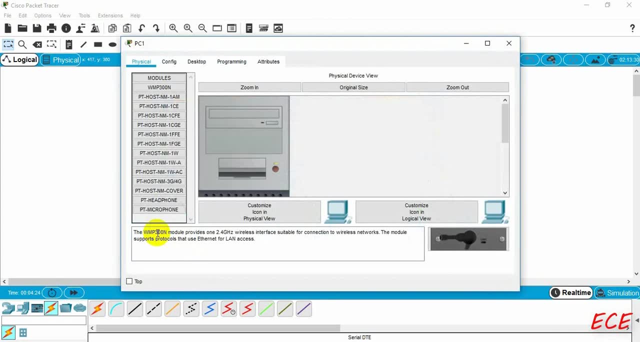 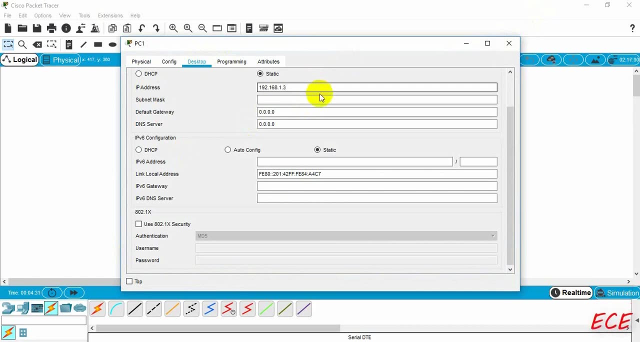 Here we are using our second device. Ok, And the gateway- default gateway- will be the same as router's IP address, because that is the only route from where the device can send and receive data, As you can see from the figure, Let's go to the next PC and here also the host ID will be different and the default 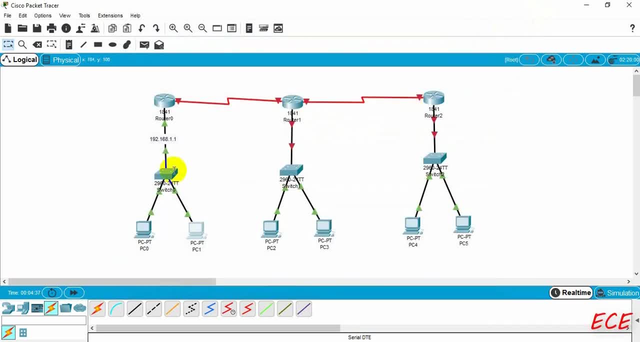 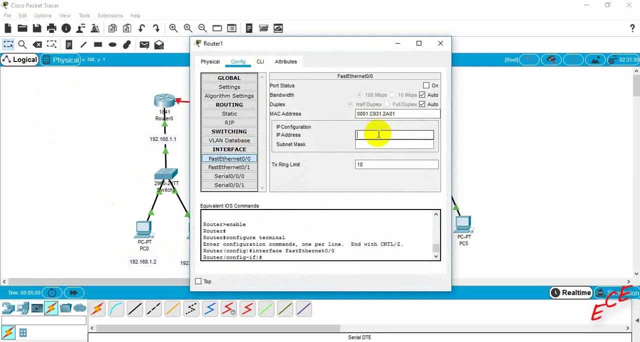 gateway will be same, And then we need to do this for the other router and the PC too. Now, let's just keep them note here, So that We will convert them later Here inside the configuration again. we need to give a IP address here, but this time this: 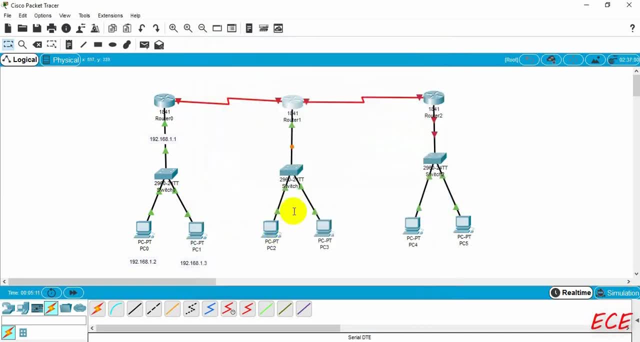 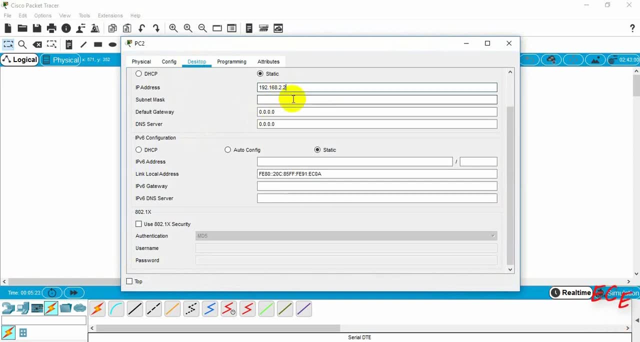 network is a different network. It's a different router. So we need to change the net ID too. We cannot give 192.168.1.. We need to give it .2345 and anything you want, but you need to change the net ID here. 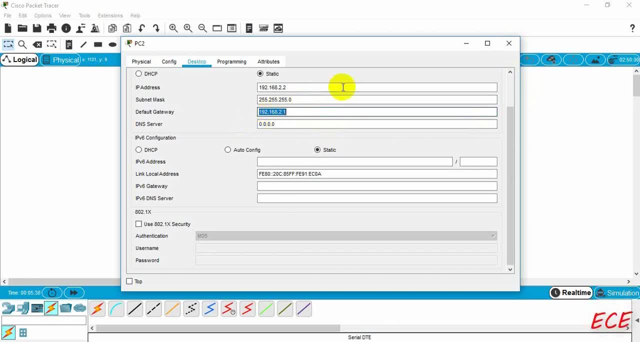 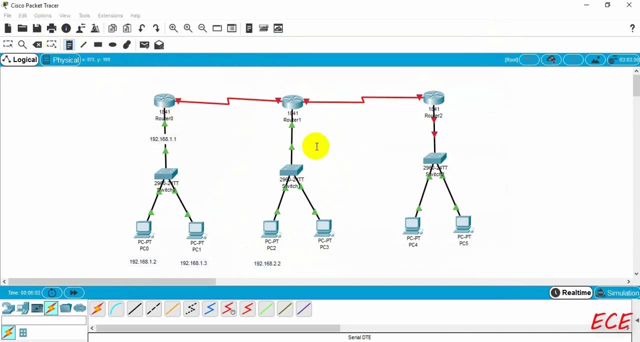 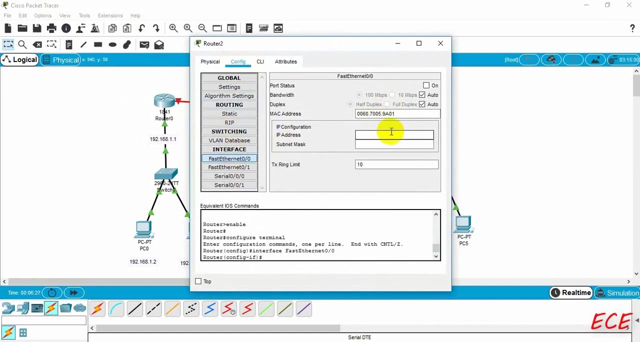 As it was our class C IP address. So you can change the first 24 bit as you want. Only the last 8 bit was for our host ID. that is why we're giving different host ID here: 11. 2.. 3., 5., 4., 5., 5., 6., 5., 11., 11., 11., 12., 10., 11., 16., 18., 19., 19.. 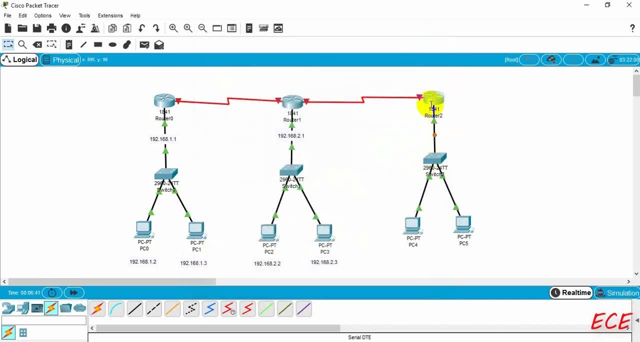 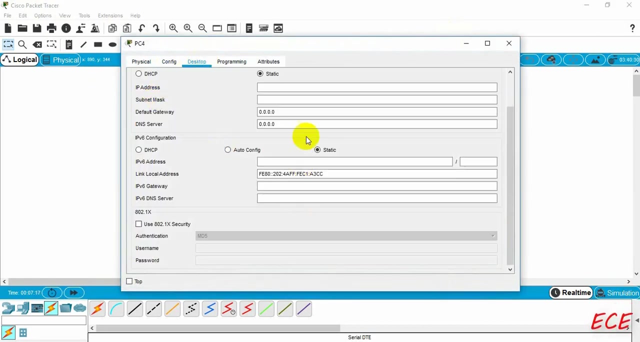 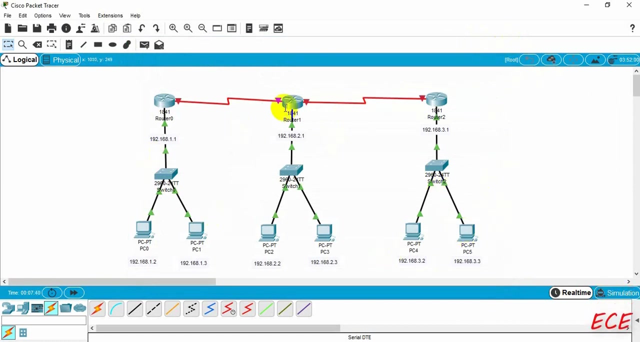 This time too, we changed our net id to .3, and then the host id was .1 for router and the pc will be .2 and .3.. Now all the things are configured. only these routes are actually not configured yet. So let's go back here again. 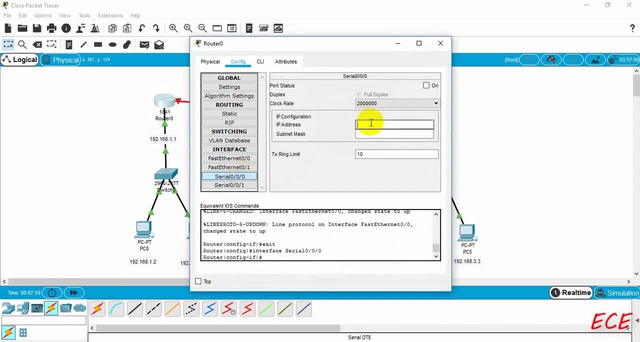 This was connected to our serial port 0. So we need to give our ip address here, And here we will use a class a ip address. You can use class c ip address here too, It doesn't matter. I am just doing it so that I can remember where I put which id. 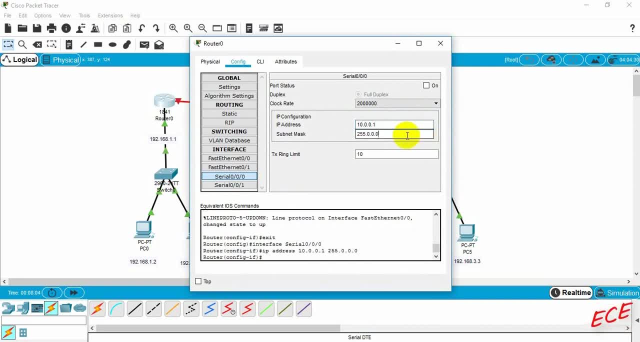 And here you can see that this is a class a ip address. So the last 24 bit will be for our host id. You can add any of the host number there. And here you can see the second router's configuration. We will add it here. 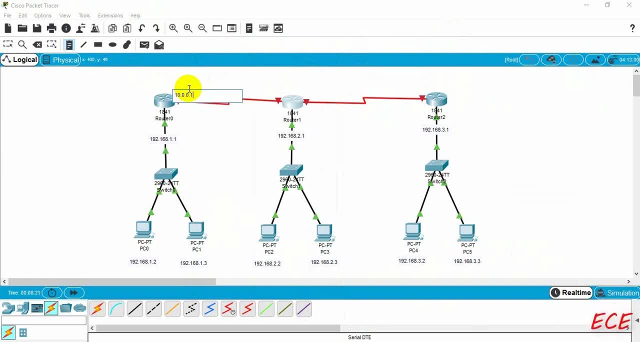 First, let's take the note here: 10.0.0.1.. And we need to give an ip address for the second router's this side, exactly like this. Here you can see that The net id was same for all the different network of a router's one side. 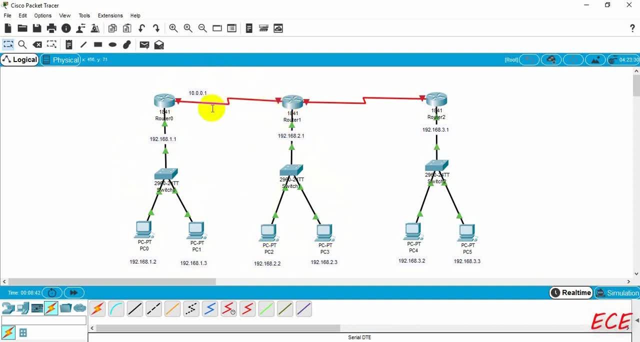 There are actually two different router, but the route is actually in the same network because in between them there are no other routers there, So this whole side will be under the same network. So that is why we are giving the same net id, 10, and then the host id .0.0.. 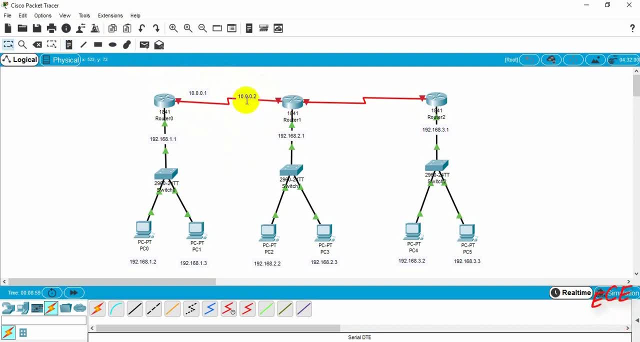 And then the host id will be different. That will be 2.. So we are giving the same net id, but the host id is different, Because this is a and this is actually inside a same net. They are both from two different routers, but we are using the same net id. 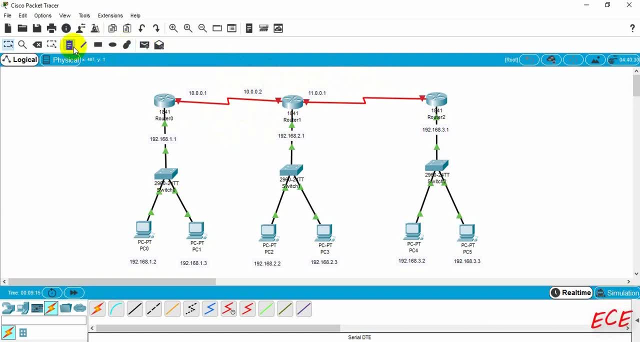 You just need to watch them carefully when you give the ip address. So let's give them this on this side. You can see this is another side of two different router again. So the net id will be same, but it will be different from the other route that we added. 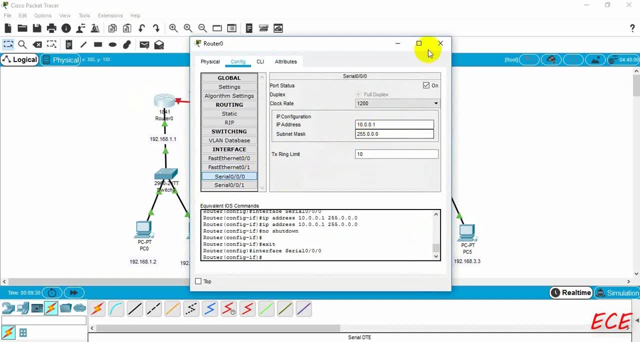 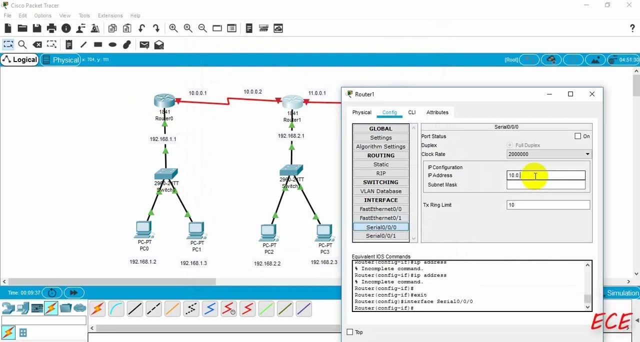 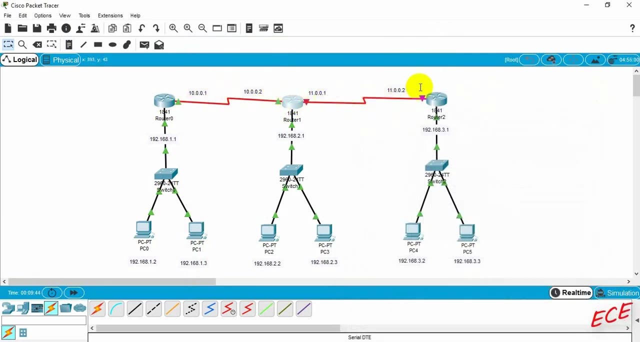 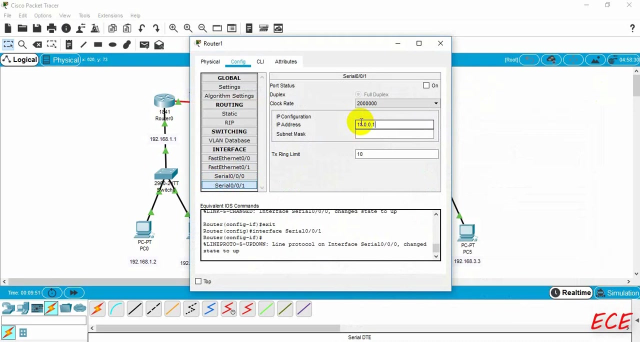 before. Okay, So now let's go to cl, port 0 and add it. Okay, So let's go to router 2 and here we need to add 10.0.0.2 and then turn it on. Now this side, serial port 0, 1, and here will be 11.0.0.1 and another side will be 11.0.0.2.. 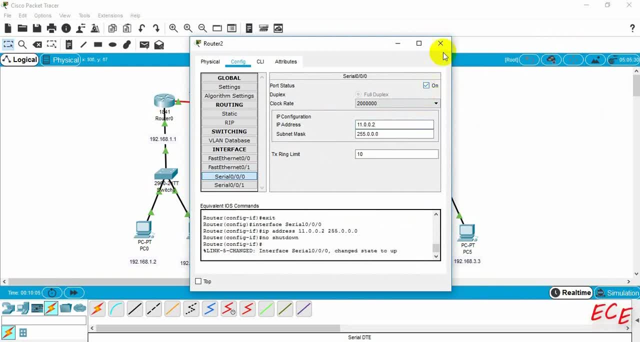 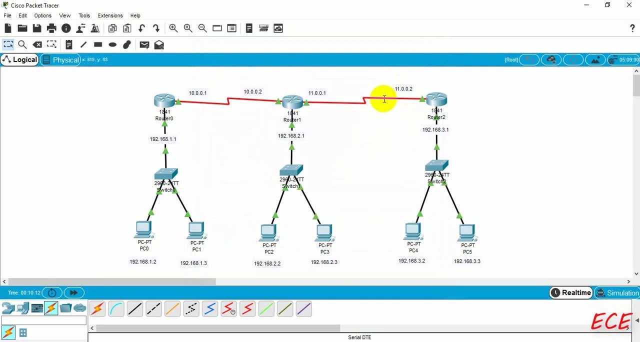 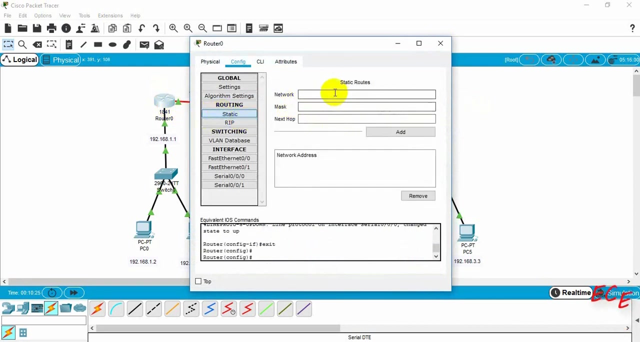 Now you will see that all the routes are actually turned on, as you can see the green mark here. Okay, And now we can just add the networks. before sending the data In the static side, as you have seen previously, we need to give network the mask and then 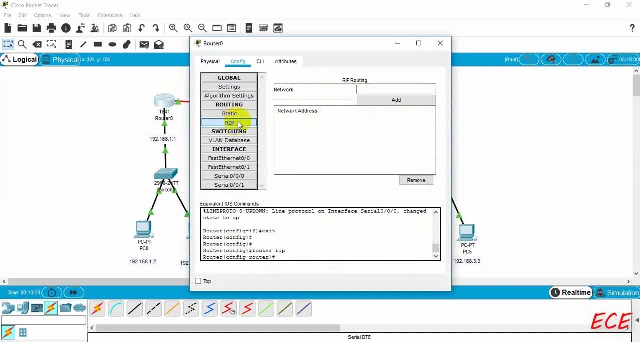 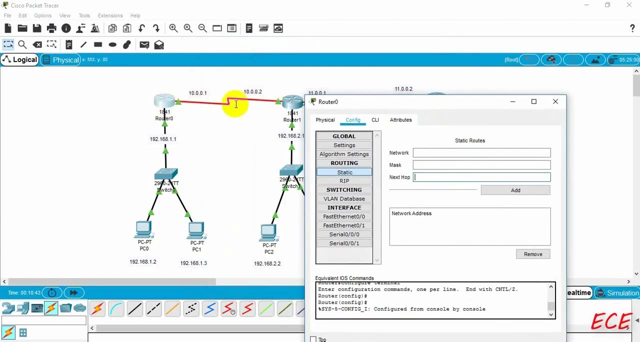 the next hop, but inside the routing information protocol- here you can see, only network is added. We don't need to give the next hop or the route name here, because this is actually dynamic routing, so here it will actually find the hop by itself. We don't need to give them the hop name, but we just need to give them the network and 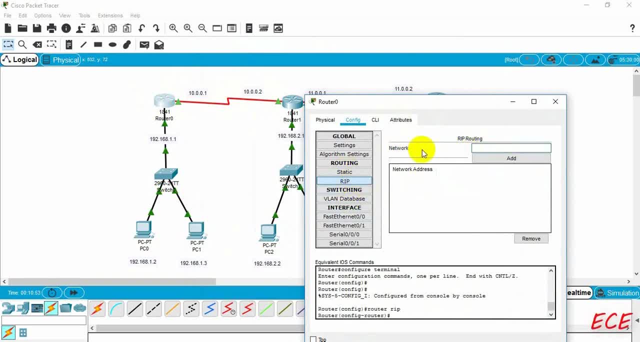 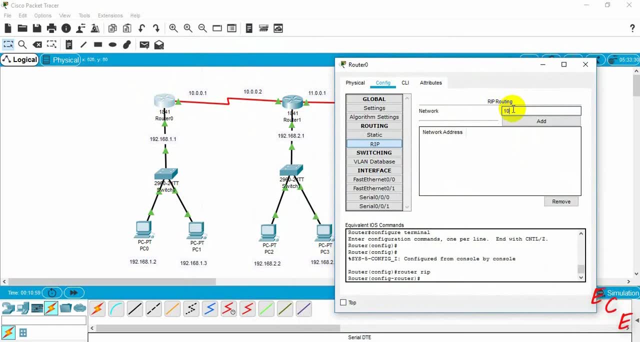 it will find the best path available for it to send the data from one device to another device or from our source to our destination. It will find the path itself. Okay, It will also find the best path available In the static. you cannot actually do this. 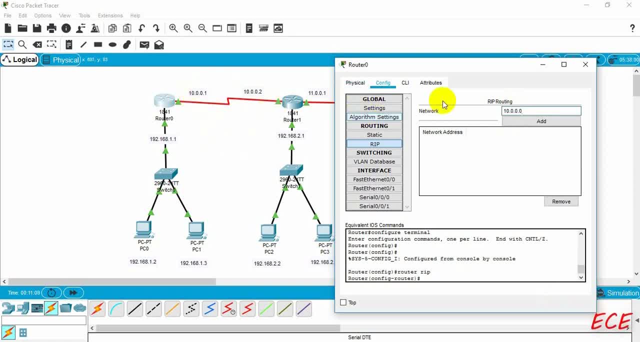 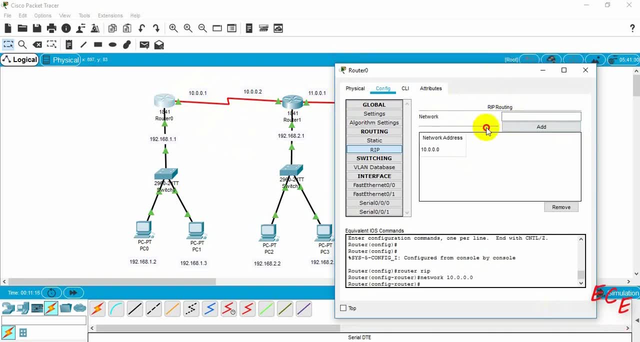 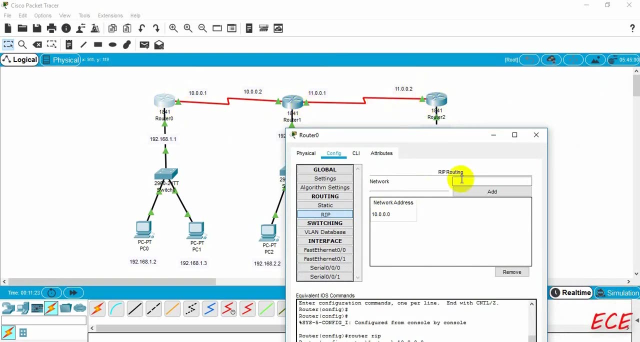 You will define the route and data will be sent from that route only. If you delete one route, the data will not be sent from the other route, if even there is a route outside the route that you have actually stated. But in dynamic you will see that if we cut one route, the data will be still sent there. 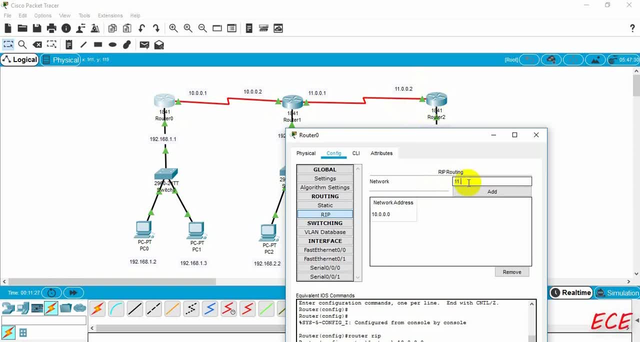 by the other route. even if we don't tell them that you can go from this way too, It will configure it itself. And now you can see we are adding the networks From router one. we can go to the network beside it and then the other route. 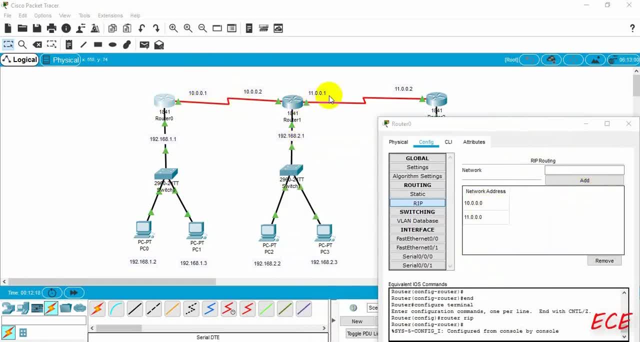 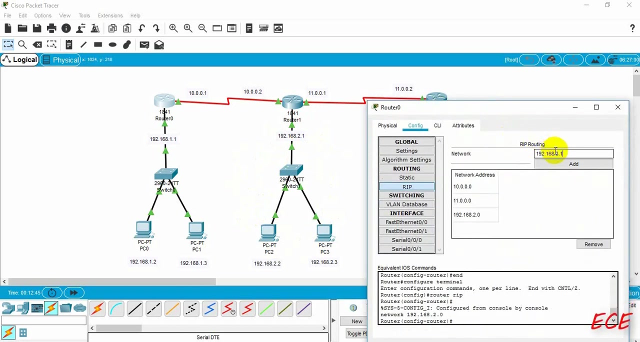 So we are adding those two, and then we need to add the separate networks of the end devices or the PCs. So we need to add them. Let's add it 192.168.2.0.. And then here 3.0.. 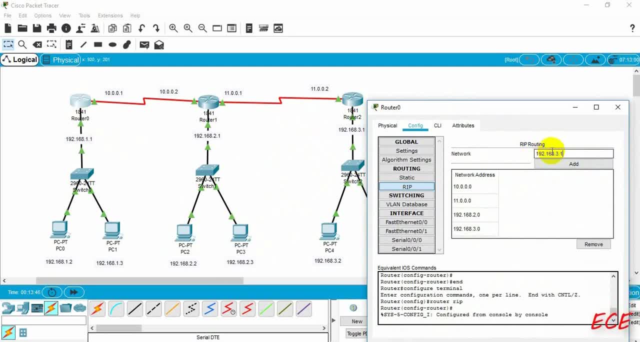 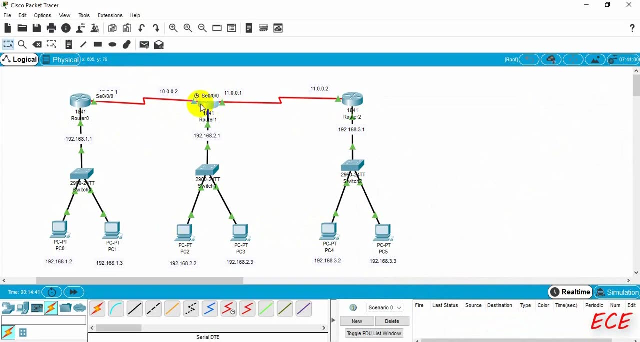 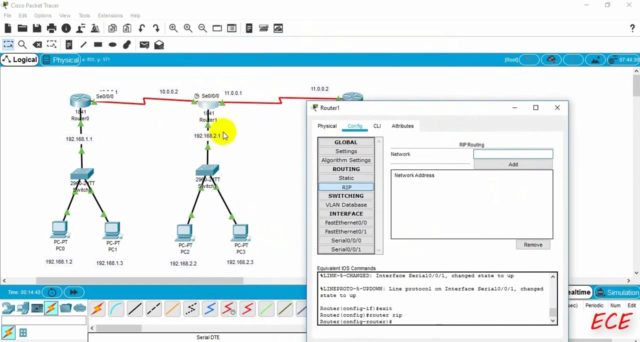 We can access any of the device from this network if we use .0, and then its own network too. So here we are sending from PC0 to PC4.. Ok, let's go to RIP again. The data just failed again. Ok yeah, I just sent the network address only on the router one, but router two and router. 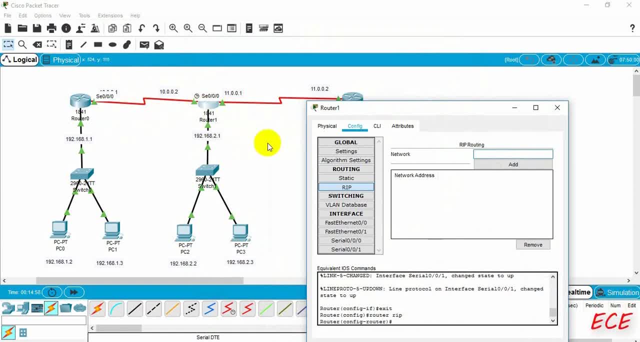 three are not configured yet properly. We did not add the network here, So let's add the network. From router two we can go to 10.0.0 and 11.0.0, and then from router two we can access the. network in the under the both the routers. So from 3.0, sorry, to 3.0, then 1.0.. Here, from the third router also, we can access 10.0.0 and then 11.0.0, then the first router's. 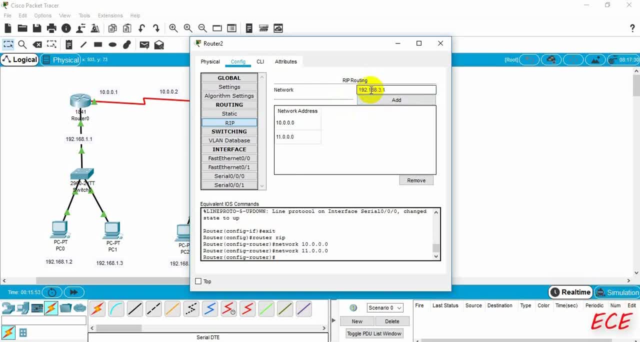 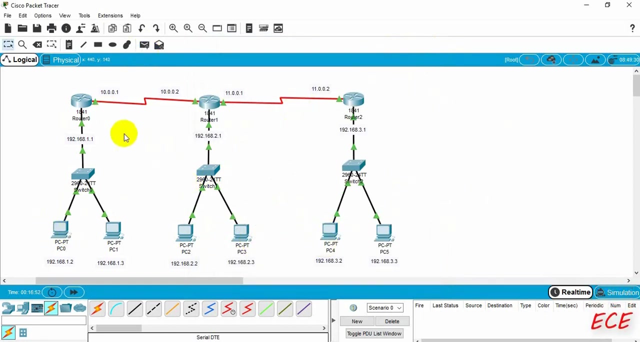 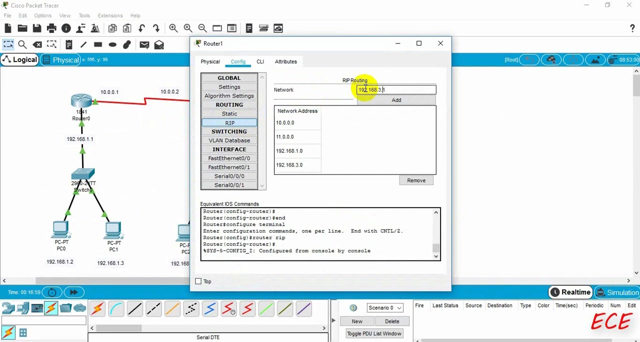 network and the second router's network. Now, if we send from here to here, ok, it failed again. ok, I did not add the network of the router's network itself. I need to add them too. So 2.0. I did not add this network, I only added the other router's network here. but I need 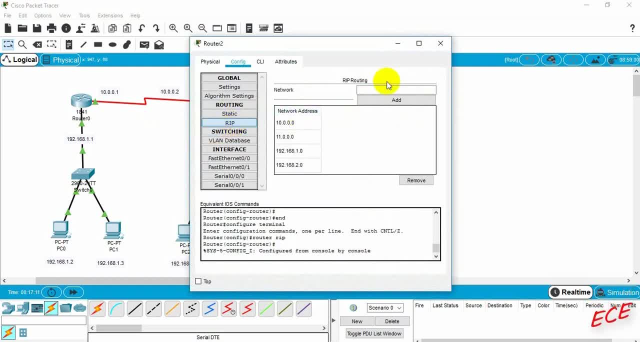 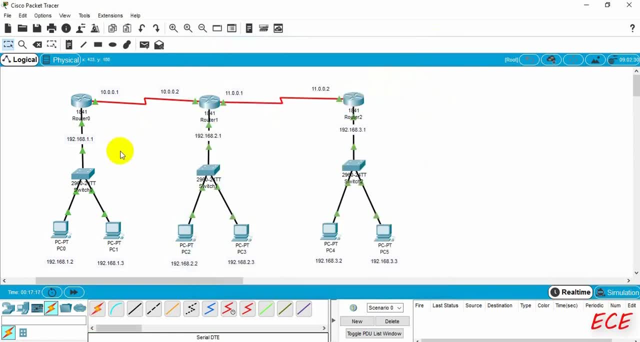 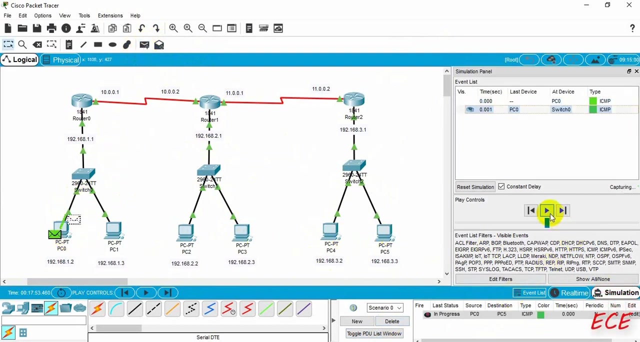 to add its own network too. Ok. Ok, Now it can fail the first time, because you can see that sometimes we can ping the device and it will take more than one minute to ping the device The first time. it happens sometime. Ok, now let's just see. 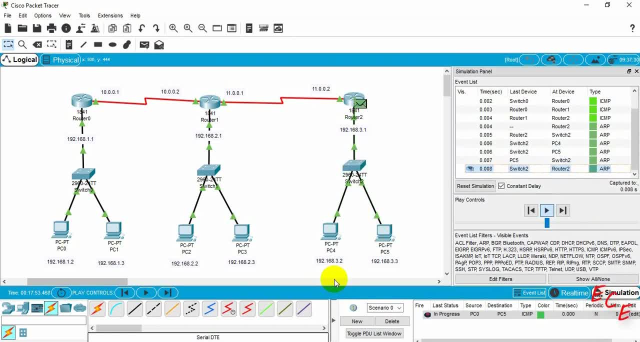 And the data need to come back to the PC0 again. It failed again. Let's send it again and let's see. Ok, Let's see how it works. Ok, Let's see how it works, Let's send it again. 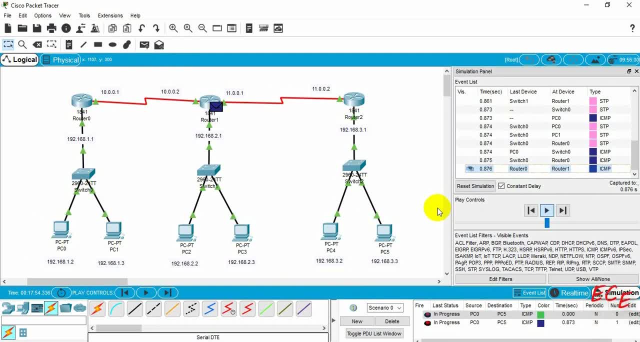 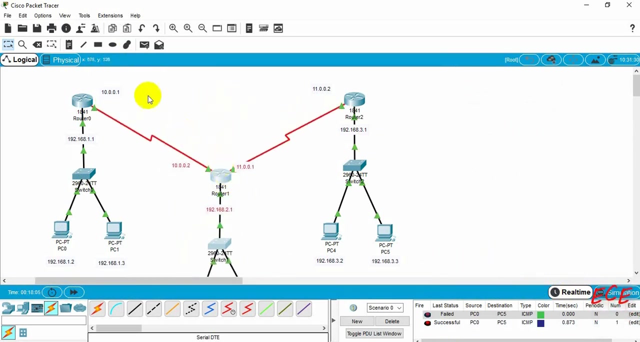 It has failed again. Ok, Let's see how it works. Ok, This time it is not working, Let's go back and we can see. Ok, Okay, this time it just. yeah, it was successful this time, All is done. but this time we will add a different network here. 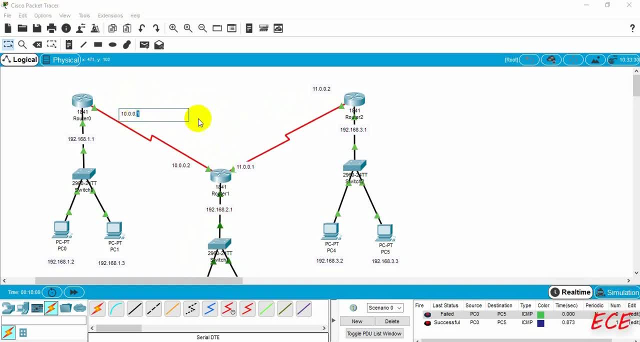 We will connect our router 1 and router 3.. There will be another route and you can see that if we want to send from PC0 to PC5, there will be a shorter route than the one given previously Here. now we can use this path from PC0 to PC5. 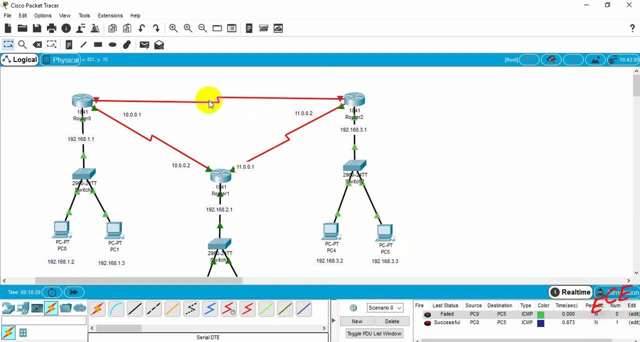 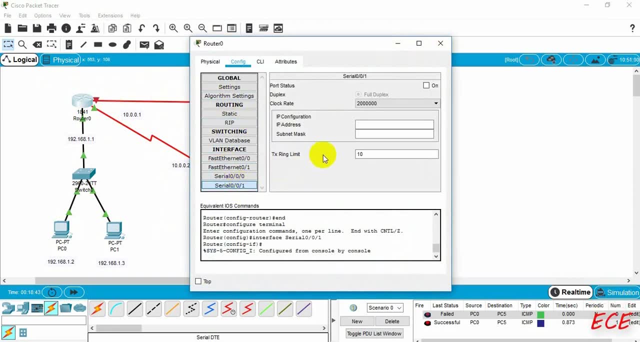 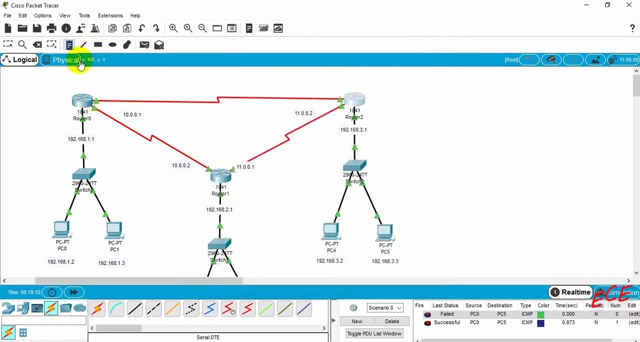 This will be actually easier than the one with another router. So here IP address. We are giving a different netID here, 12, but it will be from the A class IP address 12.0.0.1 to first router serial port 01.. 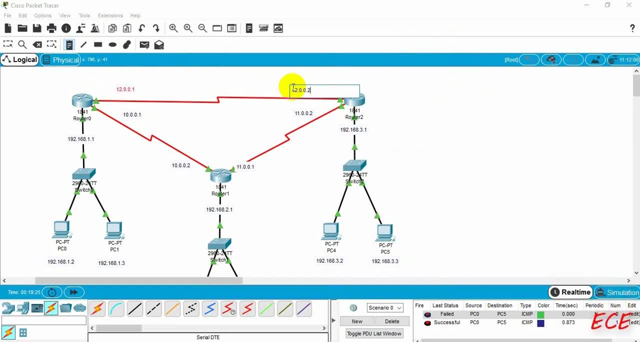 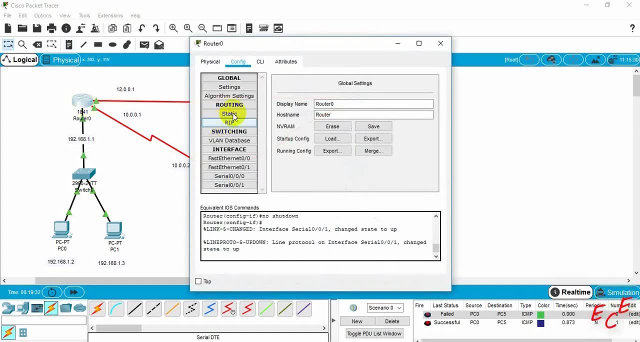 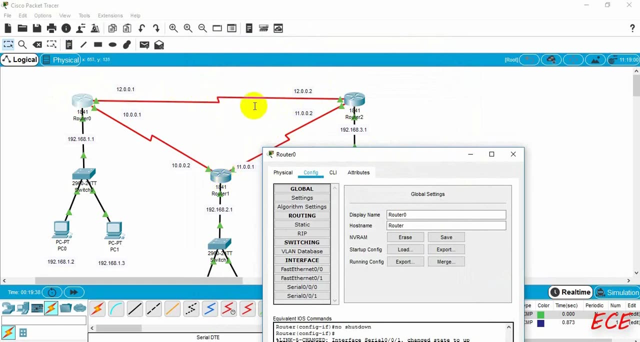 here 12: dot 0, dot 0, dot 2. so this is our another network and let's add this network to all three of them. here in the second router you can see that there is no connection with the second router to the route 12, but we will add these two. you will see a bit. 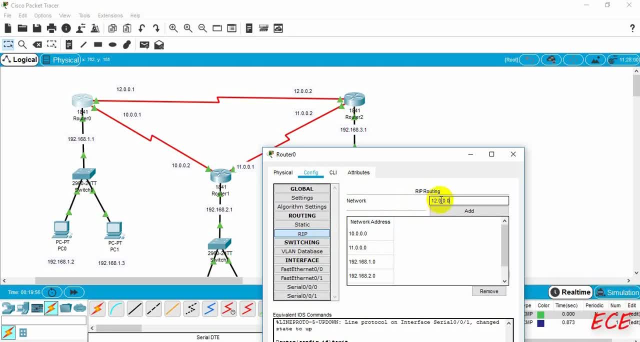 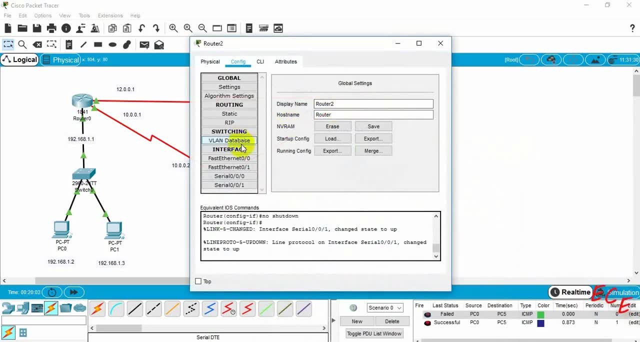 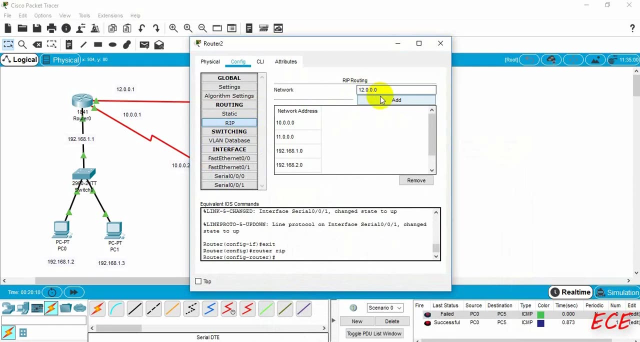 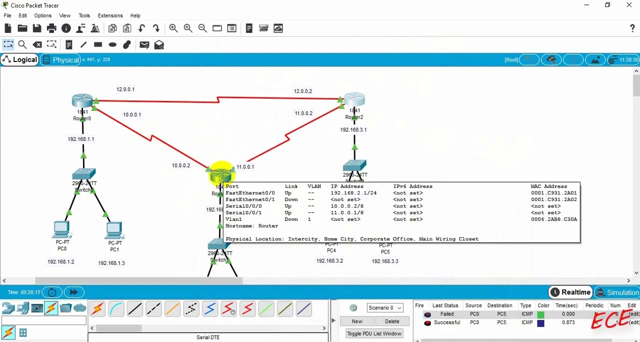 later that it is actually necessary here. let's add it to the first router and then go to the third router and add it, as they are both connected with this route. now, as you can see that here is our network, and if we, if we disconnect one where from this, this one or another one, then 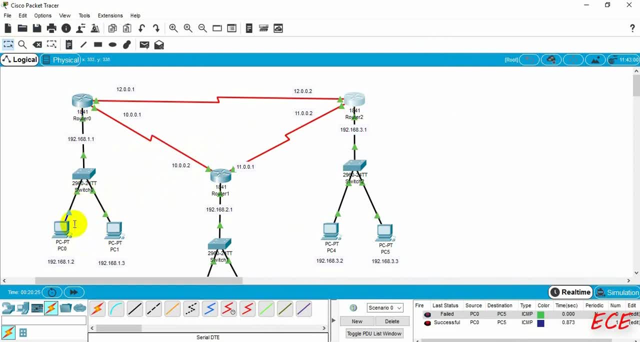 you can see that there is no connection with the second router to the route 12. you will see that we can still send data from this PC to the second networks PC or third networks PC and this there is another way to send the data. so if we 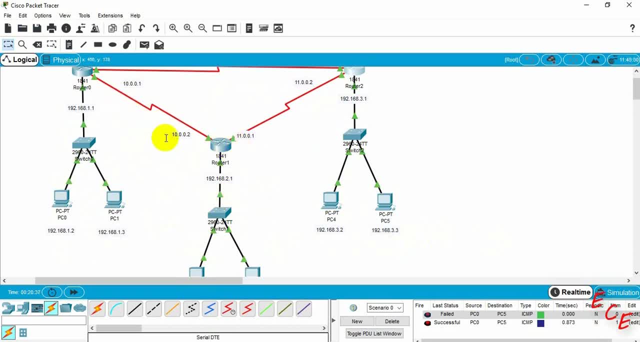 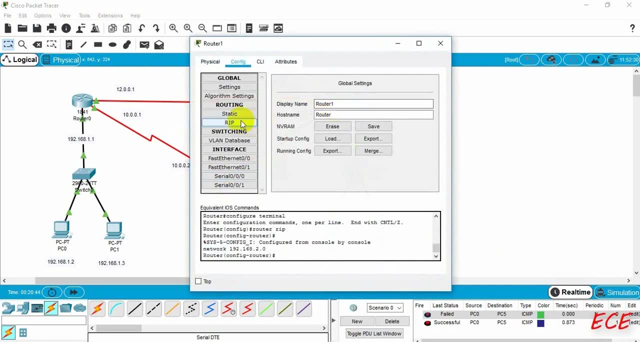 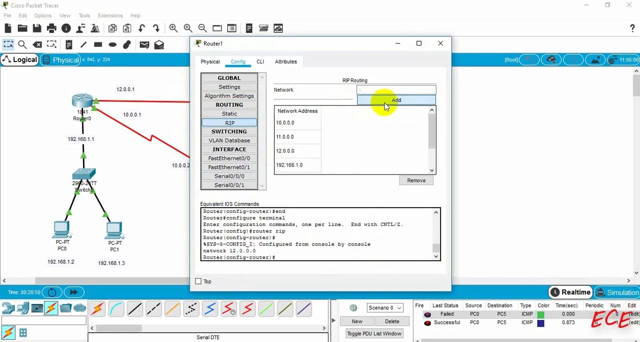 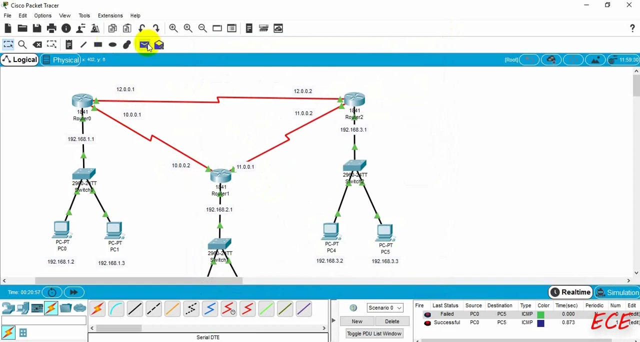 want to access devices from the second routers network, then we need to connect all the network inside this router to. so we need to include twelve dot zero dot zero inside this second router to, and if we don't do it, then we cannot send or receive data if we disconnect this. so let's send the data. 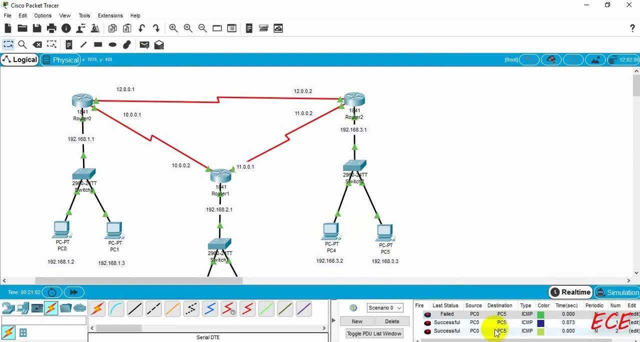 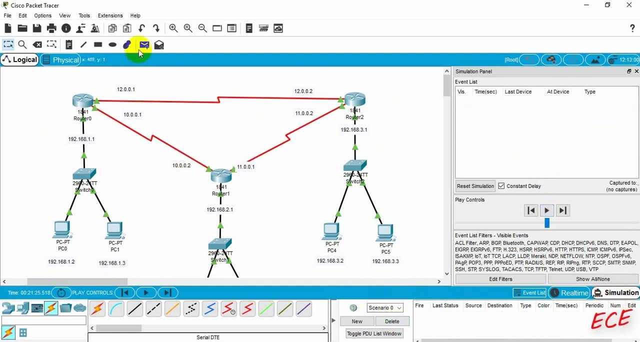 from this PC to this PC and you will see that this time it will actually take the way that is shorter there. you can see that it did not go from the to the previous way, as it was going a bit ago, but now it is actually taking the new route because it is the. 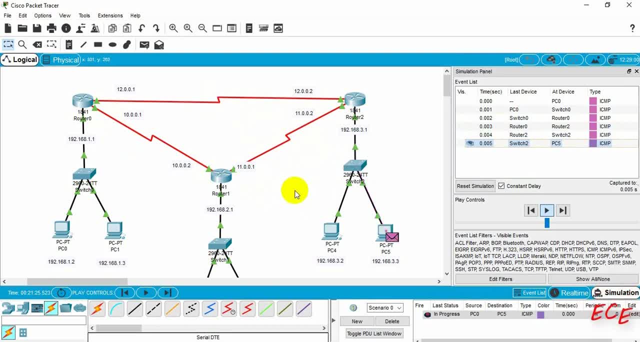 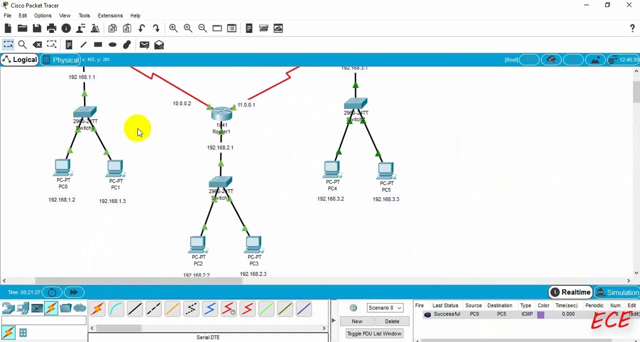 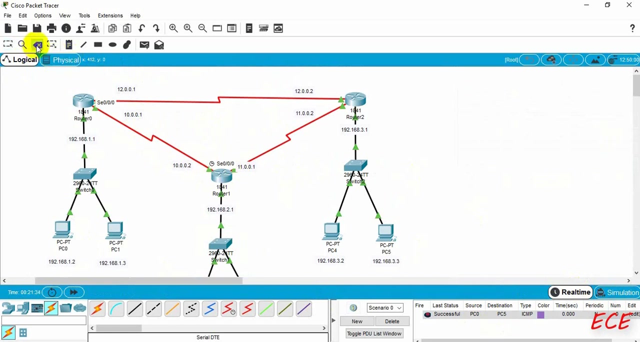 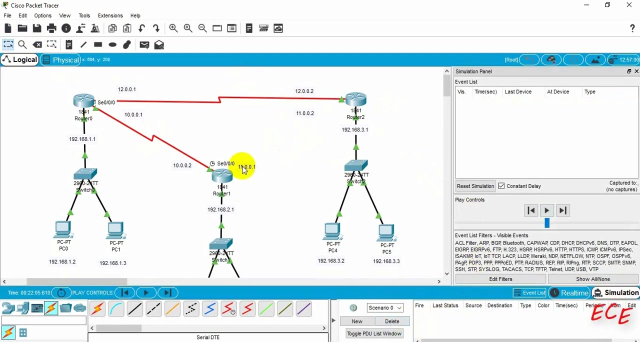 shortest path and the best path available. okay, it is successful. so now let's disconnect one where and see if it's then the data. if we can send the data, let's disconnect this one and let's try to send data from our second routers network to third routers network, because there are no direct connection between. 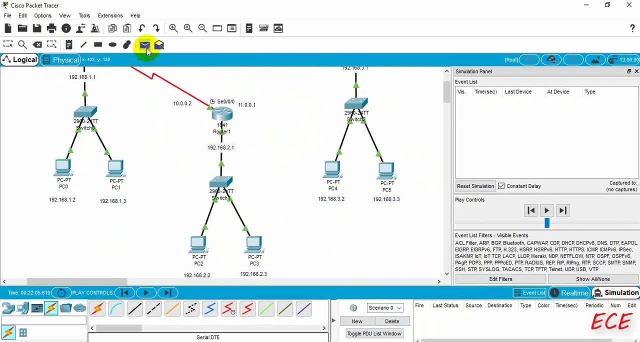 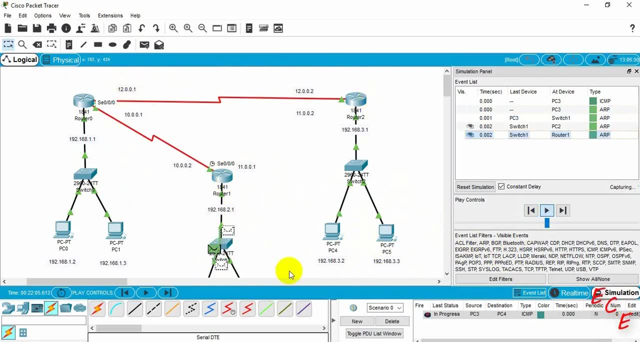 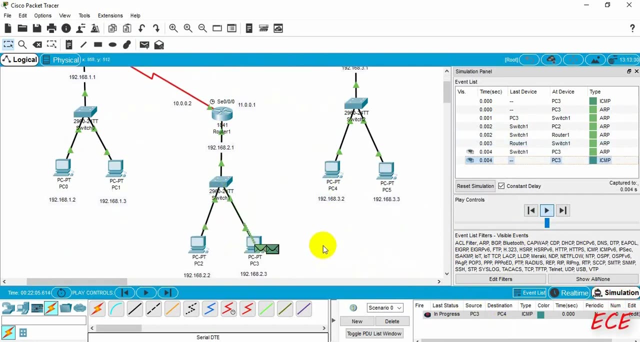 these two router, but it still can send data. you will see, let's send from PC 3 to PC 4. as I have told before, if we send the data for first time, it can actually create a bit problem. as you can see, it is coming back and then going back again. 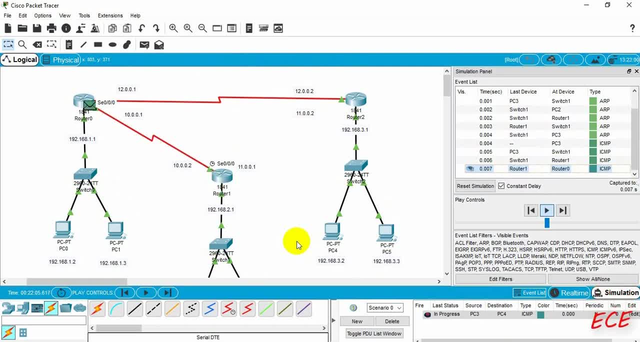 there you can see the data is actually sent using the route available, so we don't need to declare it like that. we just need to include all the network available in one network in the routing table, and we need to update the table every time we change something, as one of the route is disconnected, so the 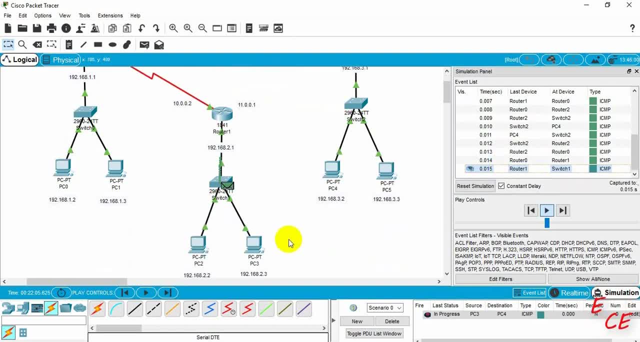 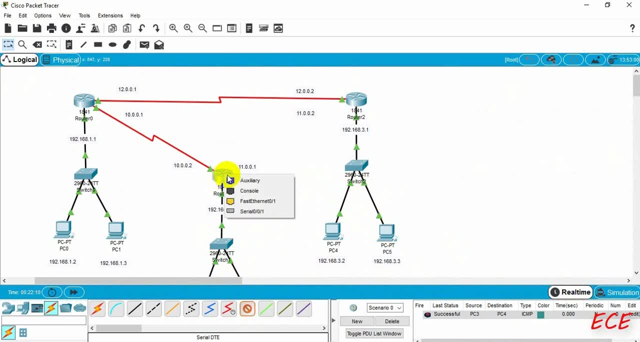 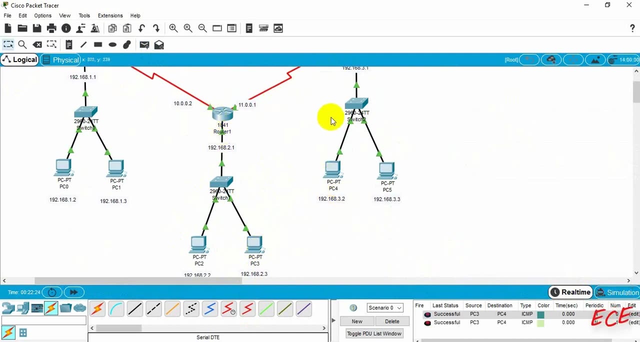 routing table is already updated. that there is only a route available is the 12.0.0, so it is using that route. this is the advantage of using RIP routing information protocol. that's all for today, and next time I will show you how to do the exact same. 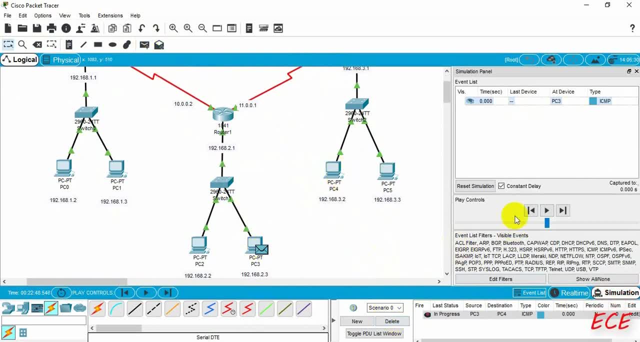 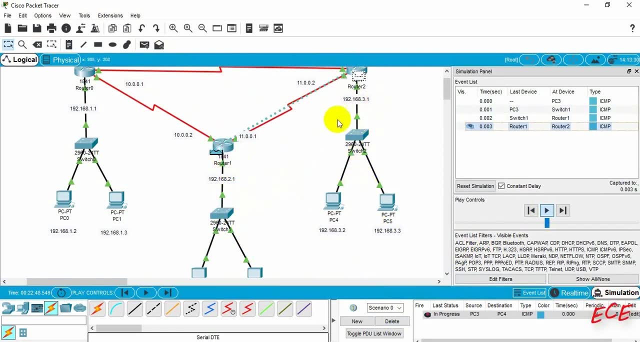 network same, this same network with a static routing. and you will see that in that static routing we cannot actually the router will the data, will not actually use the shortest path, it will actually use the first network that we will provide them, so that static routing is not actually the smartest one, but RIP. 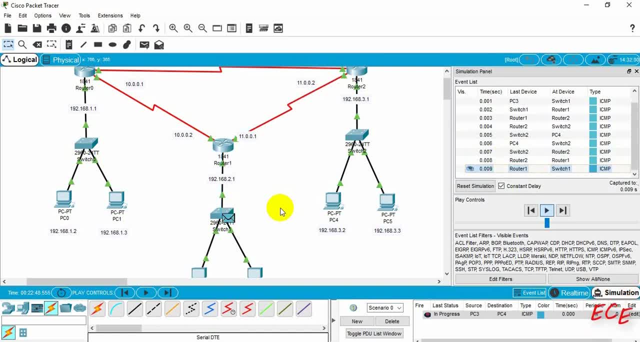 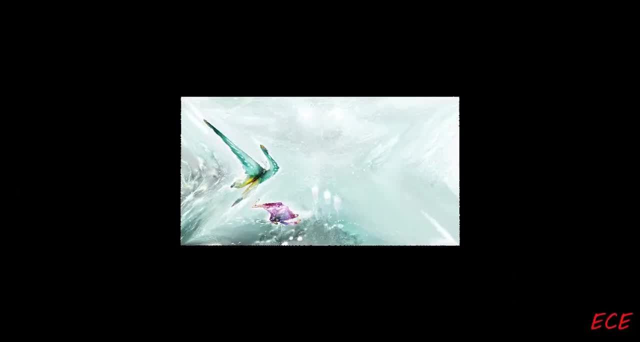 is actually really smart because it can actually understand the best path using hope count. thank you for watching. 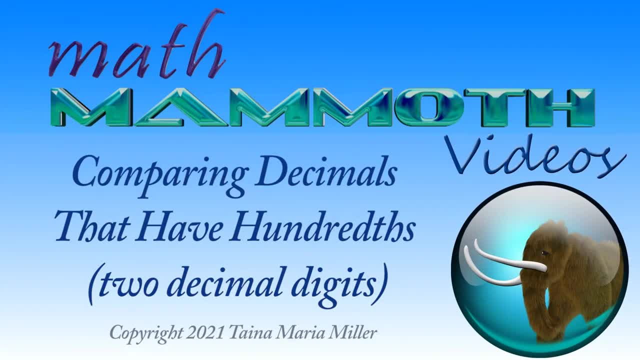 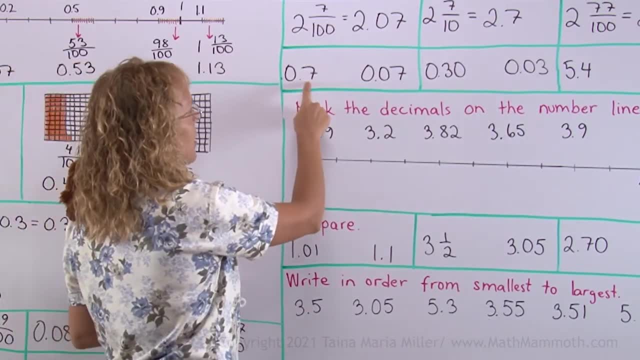 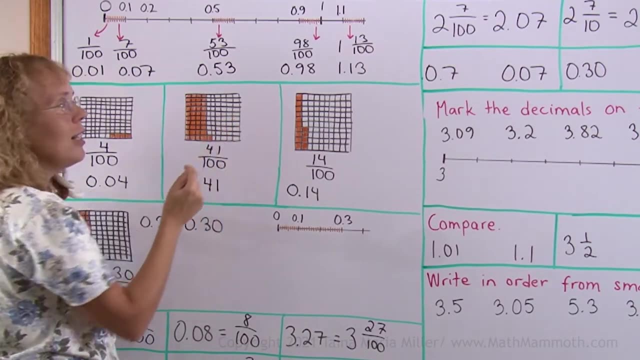 Here let's compare a little. Which number is more: 7 tenths or 7 hundredths? Well, that's an easy question, isn't it? If you colored 7 little pieces here, that would be 7 hundredths. 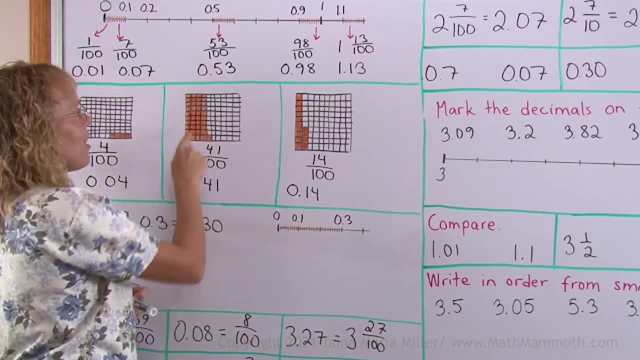 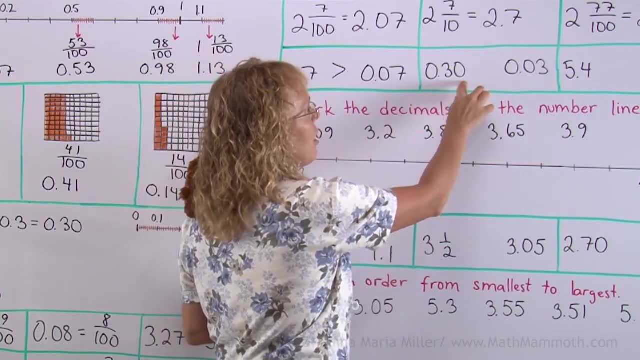 But to color 7 tenths I would have to color 7 whole columns, so surely that is more. You can think the same way here. Here's 30 hundredths and 3 hundredths. Well, it's easy, 30 of course. 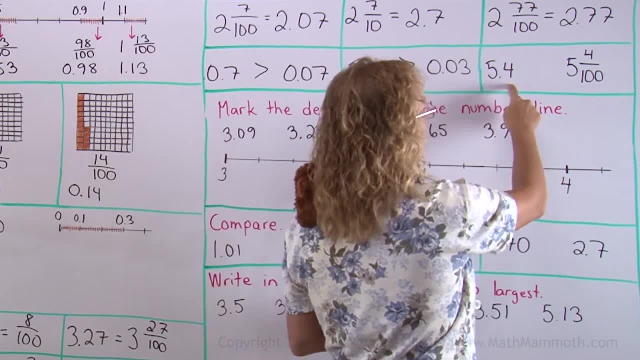 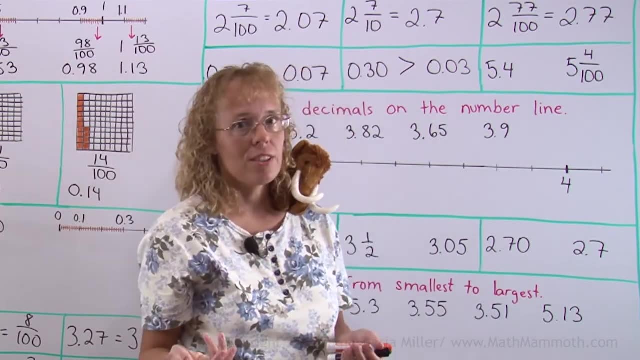 is more than 3.. And then 5 and 4 tenths, 5 and 4 hundredths. The question is, which one is more, 4 tenths or 4 hundredths? And again you could use this and reason in a. 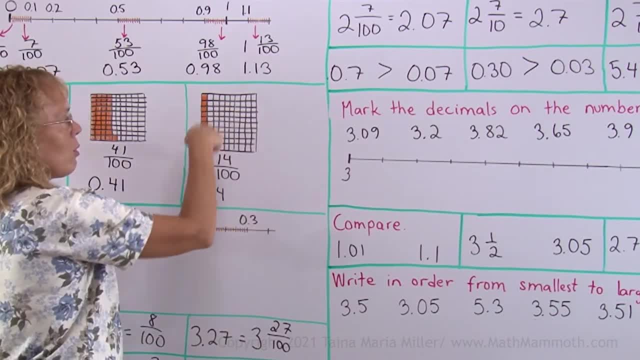 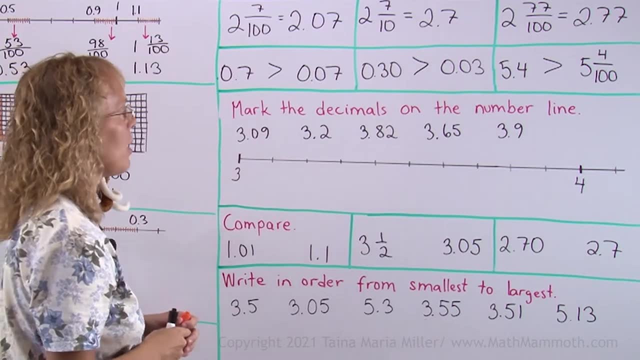 similar way, 4 little pieces is 4 hundredths. 4 whole columns would be 4 tenths. so that is more here. Now we're going to mark the numbers. Mark the decimals on the number line. What is it Matthew- Oh, Matthew- is asking for?